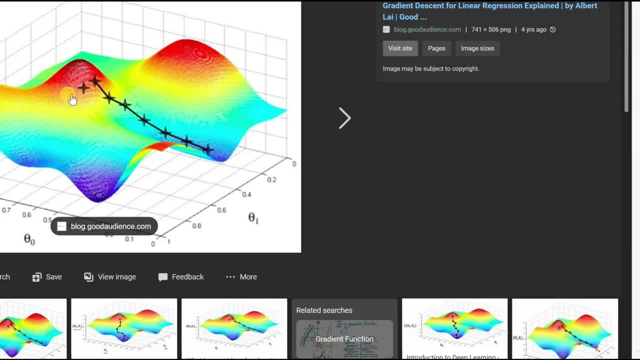 used in machine learning and deep learning to train models. Now, the goal of this gradient descent is to, you know, find the optimal value of the model parameter that minimize the difference between the the predicted output and the actual output. So it worked by computing the gradient of the cost function with respect to parameter, with 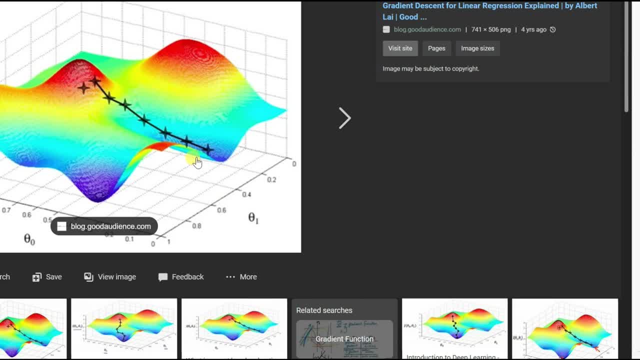 I mean, which represent the direction of the steep and decent that you can see. this is like a peak or it is moving toward the steep and decent. This is the, you know, lowest point. So that is what we want to reach Right. lowest error. okay, so so that the algorithm you know start with some. 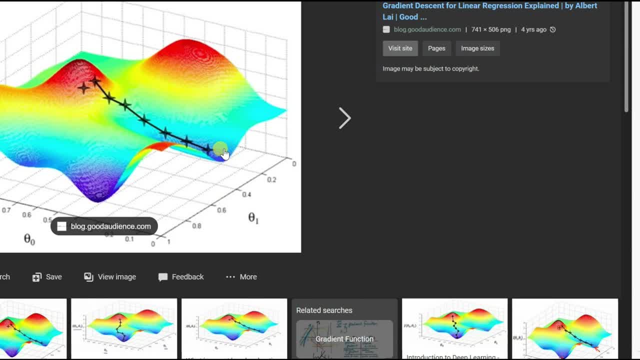 initial value of the model parameter and iteratively update the parameter by taking a small step with the help of, you know, learning rate that we have learned, okay, so in the direction of negative gradient. so the size of this tape is controlled by learning rate, like I told you, which determines how quickly the 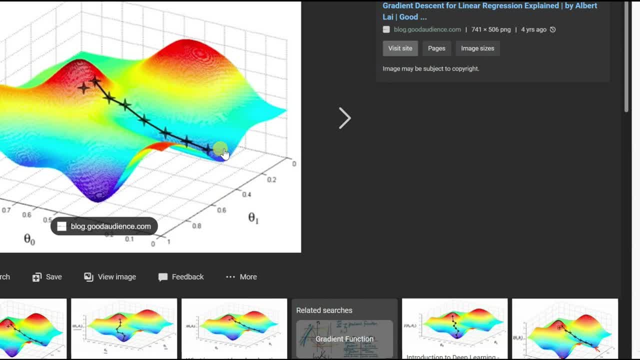 algorithm converts to minimum or you know cost function. so this process continue, you know, until algorithm reaches a minimum, at which the point other parameter are considered to be optimized. so the minimum can be either a local minimum or global minimum, okay, and depending upon, you know properties of 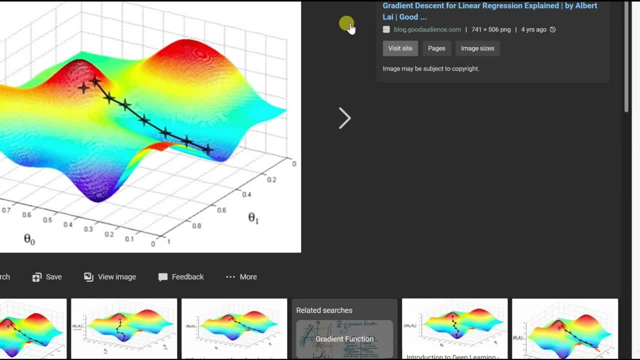 cost function. I mean we found, so I mean we'll see that later in, you know, I mean you can even see in machine learning tutorials. I have, you know, explained it, you know in better way. so, moving towards, so, yeah, so that is what we are going to see in the next video. Thank you for watching. 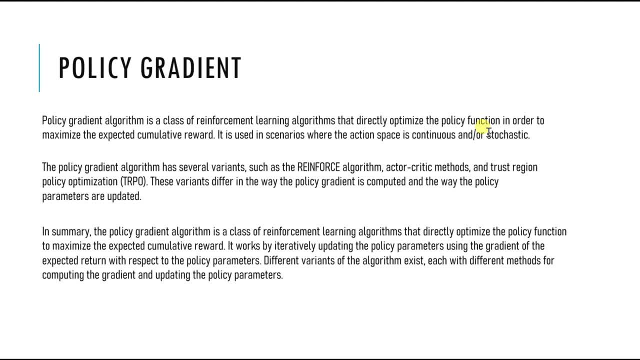 you know this policy gradient is, I mean this stochastic gradient now. so policy gradient algorithm, you know, can be classified into I mean on policy and off policy algorithm. so on policy algorithm, such as reinforce actor to critic. so basically what they do? they update the policy using current policy experience. 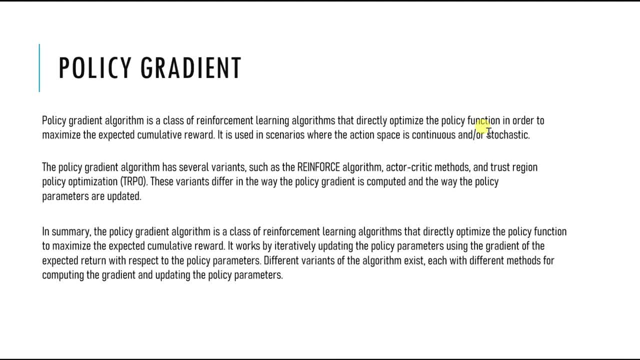 while off policy algorithm, such as you know, td3, DPG, etc. update the you know policy using experience from the separate buffer. okay now this policy gradient algorithm, we have been successfully applied to wide ranges of tasks, of tasks like roboticspreparing, game, natural language. 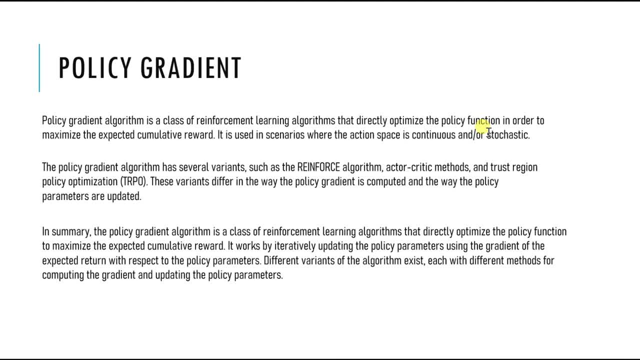 processing. now, i mean, one of the advantage of policy gradient algorithm is that they can learn directly from raw sensory information, such as image, audio, 아마, with out the need of you know, with out the need of feature engineering and, however, there can be computationally expensive, especially in cloud, in high dimensional state. 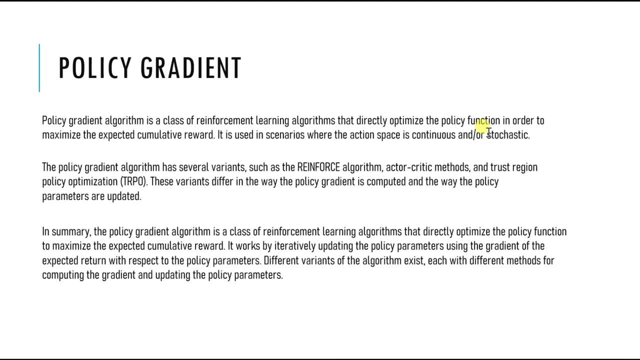 and action space. Since we have learned, learning the advantage, let's, let's see what you know more advantages of this. so basically, as far as I know- so I mean the advantages of policy gradient algorithm includes is handling the- you know, continuous action space, which means in policy gradient method we can handle continuous action space directly without. 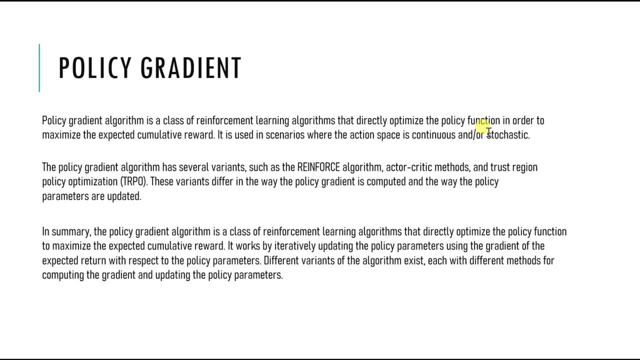 the need of- I mean okay, and which is like major advantage over value based methods such as Q learning. now it has, you know, stochastic policies also. so what that means is policy- you know policy gradient algorithm that can last stochastic policies, which can be, you know, useful in domains while exploring 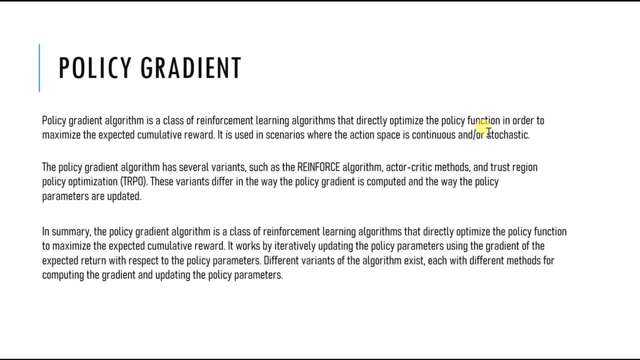 different action in, you know, important for finding. it is important for finding optimal policy, because without exploring I mean the agent will never know. now another advantage is better convergence property. so what I mean by that is so policy gradient algorithm has you know, better convergence property, that you know. I mean then any value based method we have learned till now in some. 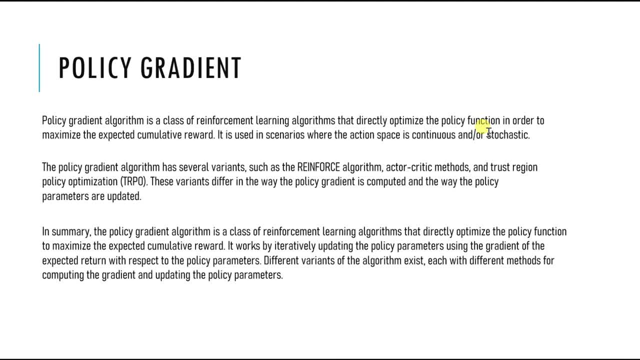 cases so, such as it high dimensional or, you know, continuous space, this policy gradient, you know, outperform any algorithm. so that is that is the main. I mean, you know, advantage. now coming to disadvantage of policy gradient algorithm includes, like, high variance. so what I mean by high variance is that 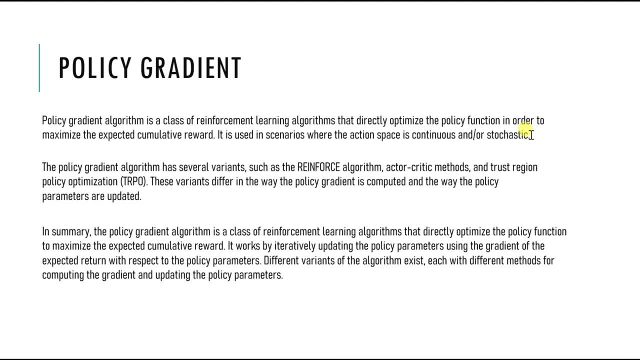 policy. gradient method can suffer from high variance. you know haziness or you can say like, which can help them slower. you know to convert compared to value based method. okay, when there is, you know I mean very disturbing data, so that time you know what happens. it learns slowly, but it. 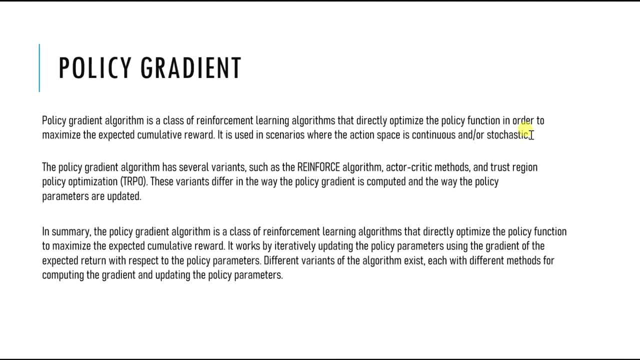 takes so much time and computational energy, and that's why you know it's very expensive sometime when the data is not- that you know- stable. now it has also one you know disadvantage: that is local minima, and so policy gradient method can converge to local optima rather than global optima, which you know lead to some optimal. 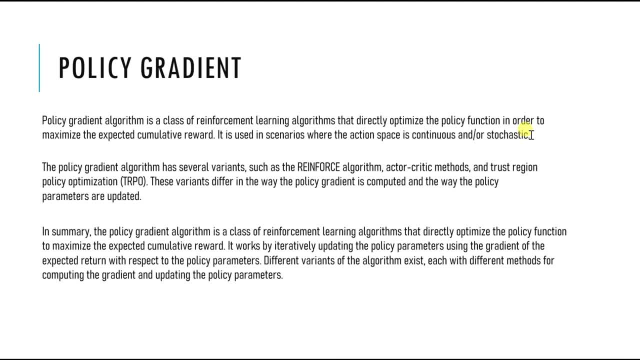 policies. so, if you know, we leave our agent till local optima, our agent will never want to learn what exactly the global optima is. okay, so until our agent doesn't reach, I mean, this global optima, I mean obviously we will not be able to, you know, achieve the hundred percent reward in I mean like 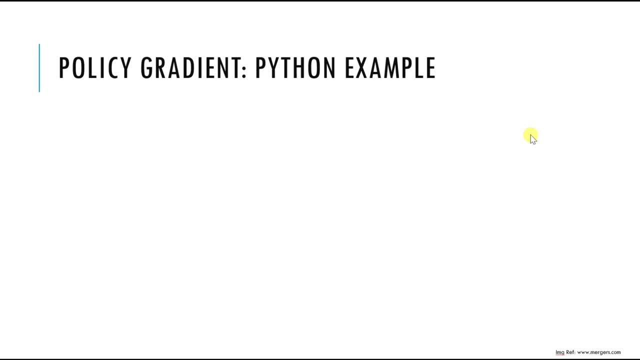 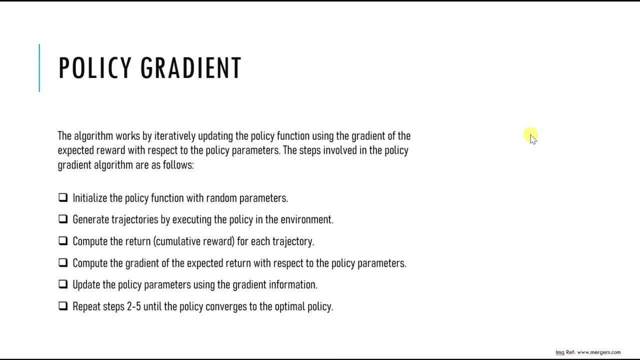 like, just think this as example. okay, now another. you know if you go to I mean disadvantage will be like difficulty in balancing, you know, trade-off between exploration, exploitation. so that is, you know policy gradient method require a careful balance between, I mean, exploration and exploitation to ensure that the agent explore enough to discover new and 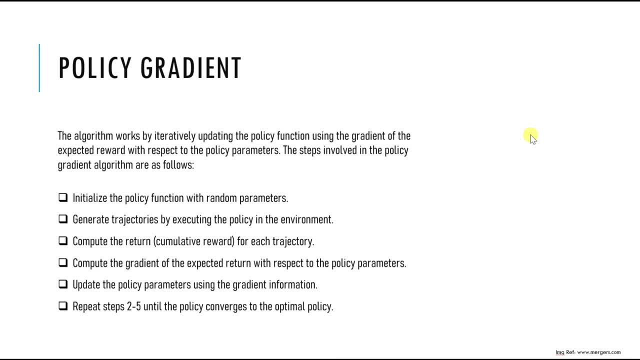 better policy while also exploiting what it has, you know, learned so far. so I mean what I mean by that is. so policy gradient method can be, you know, I mean sample inefficient, which mean they may require large amount of data to achieve in a good performance, especially in, you know, high dimensional or continuous space. 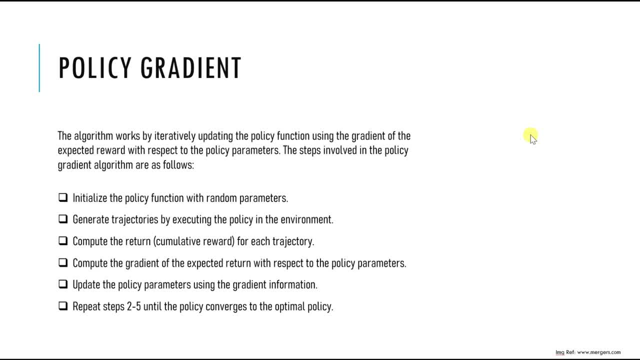 state space and that's why, you know, sometime it only able to reach local optima, not the I mean global optimum. now let's learn how basically the working is like, step by step, so in very detail explanation of you know each step that I have defined here. so basically I mean first what we do. we initialize the. 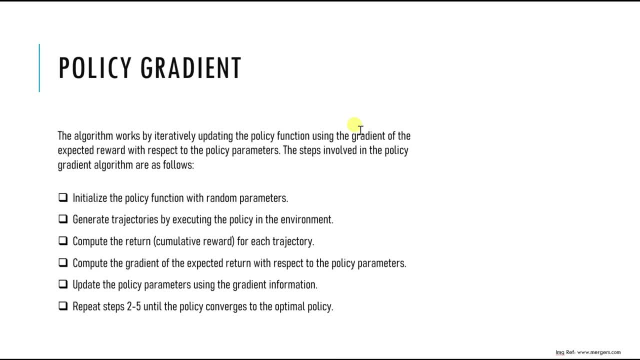 policy parameter randomly. okay, so if the policy parameter is random, then we can initialize the policy parameter randomly. okay, so if the policy parameter is random, this tape, the parameter of policy function are, you know, initialize randomly, typically using another distribution with small variance. then what we do is, I mean, we generate trajectories. okay, so in this step I mean 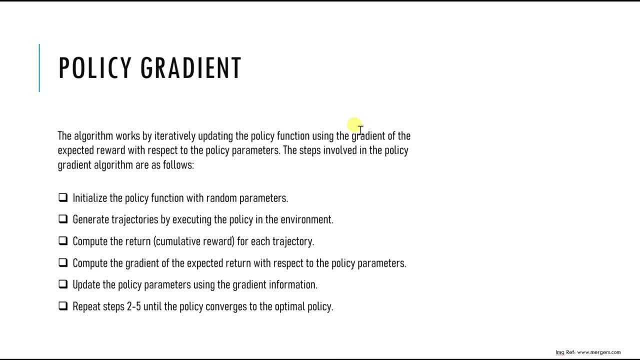 the agent following, you know, current policy in environment and collective set a set of trajectories. trajectories is a sequence of state-action pair that you know agent experiences during one episode. now, next is compute. I mean the gradient of the expected total reward. okay, so in this step, the gradient of, you know, of expected total reward with respect to